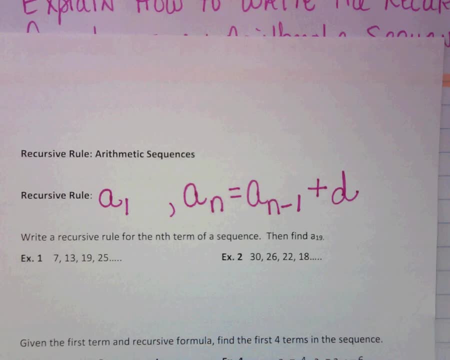 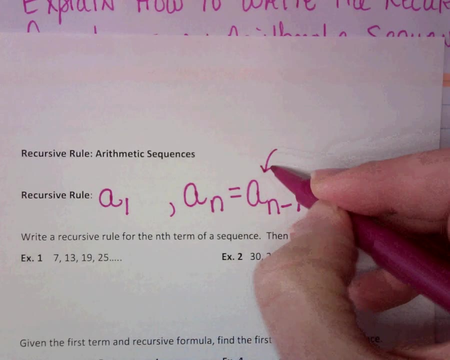 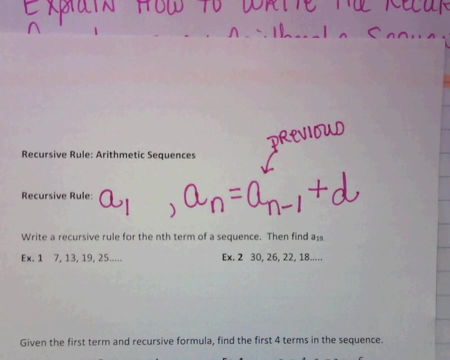 The a sub n is just saying take the previous term and add or subtract the common difference. So don't let this terminology throw you. It's just saying take the previous term and add or subtract the common difference. If I wanted to find the 23rd term, I would look at the term before it- 22,- and apply my recursive process. 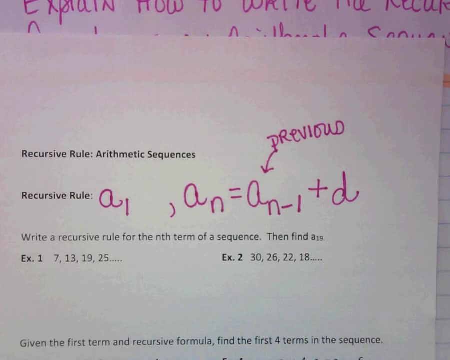 So it's a little bit different. It's a little bit more difficult. You have to know the previous term to be able to figure out the next term. So look at the first example. It says: write a recursive rule for the nth term of a sequence. 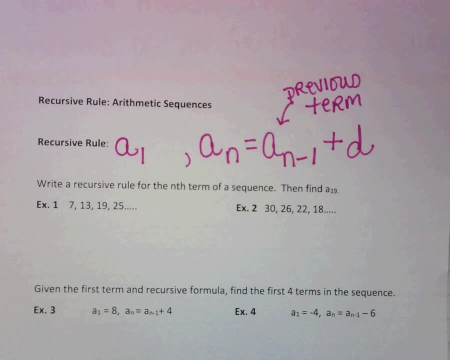 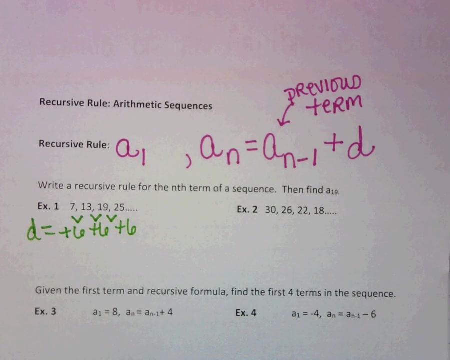 Then find a sub 19.. So the first thing we're going to want to do is find out our common difference. Every time, here we are adding six. So that is our common difference. So all we have to do now is state what a sub one is. 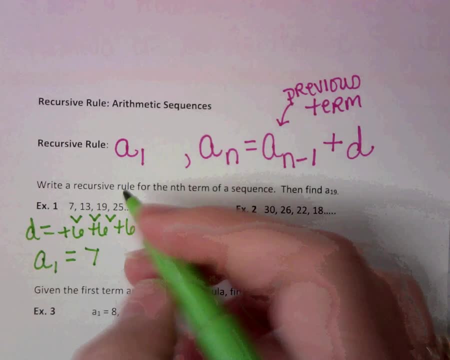 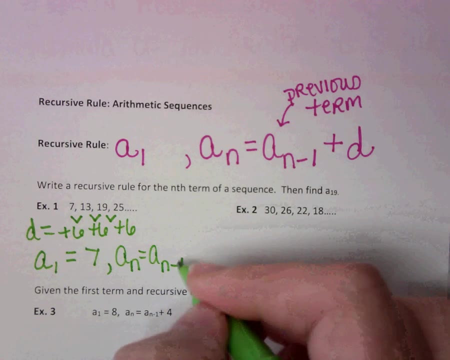 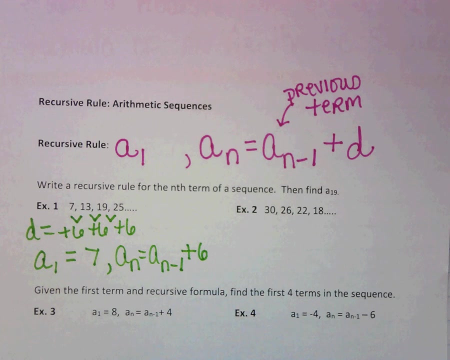 a sub one is equal to seven. Then we write: a sub n equals a sub n minus one, And then the common difference was plus d. One thing I want to point out is because we'll talk about other types of sequences later in the year. 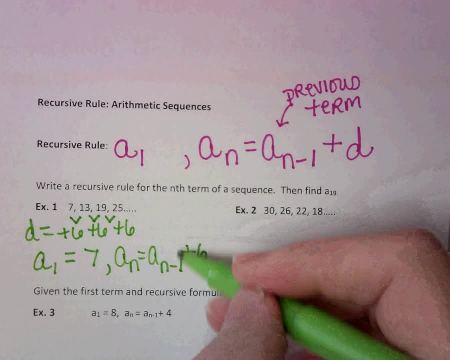 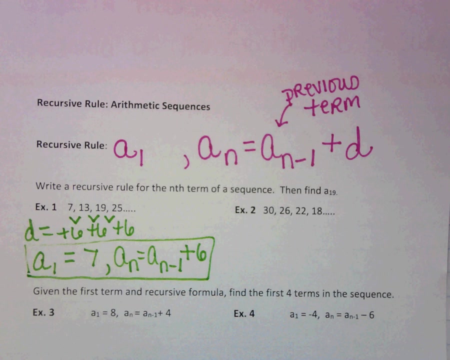 is that with an arithmetic sequence it's always plus or minus something. We're always adding something or subtracting something to a sub n minus one. That's one way to tell how it would be arithmetic. Okay, So then I want to find a sub 19.. 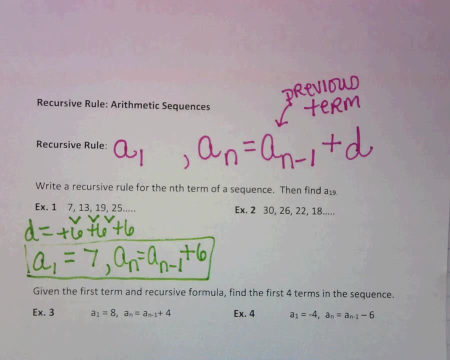 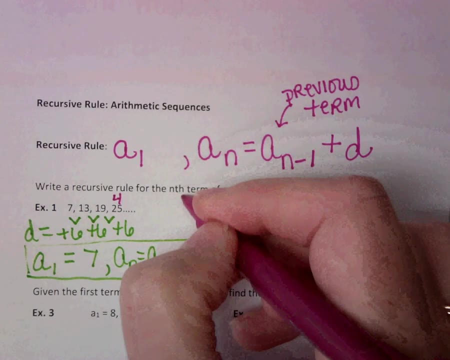 And I'm going to actually throw myself. So we know that. let's see, we're at one, two, three, the fourth term, And we have to go all the way to 19.. We should be able to see that the pattern is adding six. 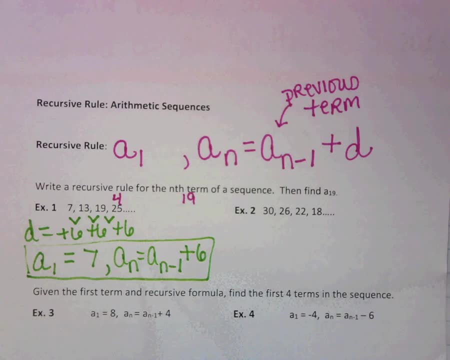 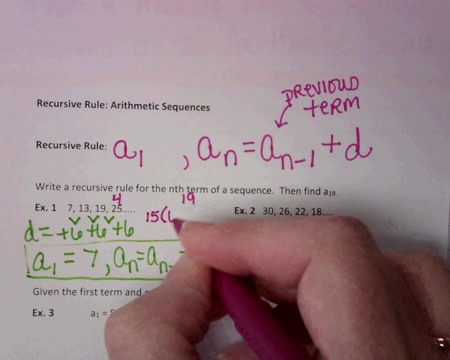 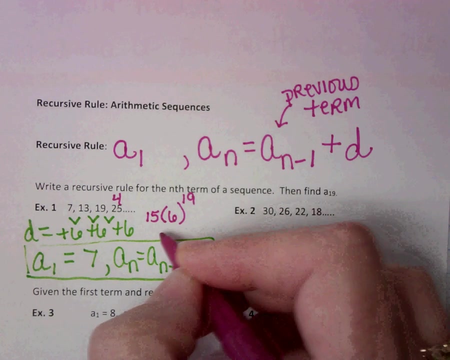 So how many terms is that? between four and 19?? That's 15, right? So if I have 15 terms and I'm adding six each time, could I do 15 times six, Which is what? 90, no, 80,, 90,, 90. 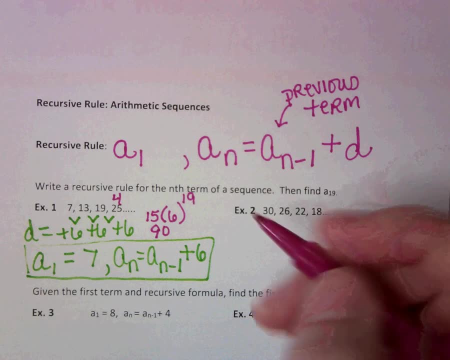 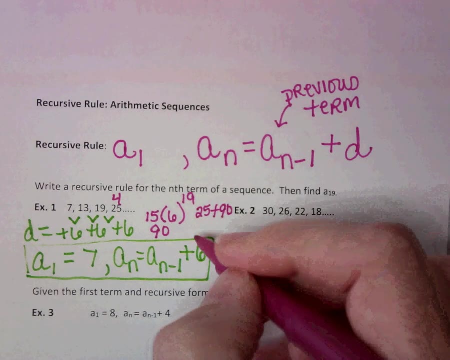 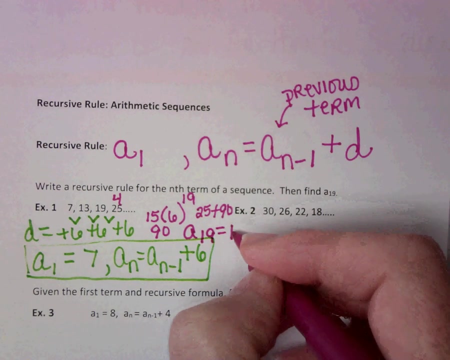 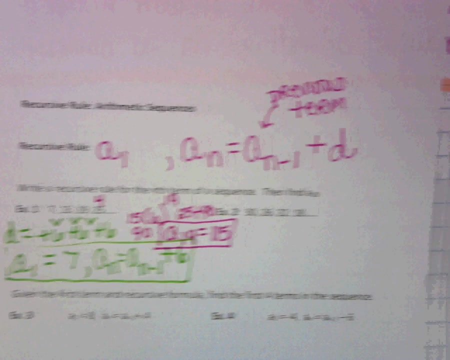 And then could I add 90 to 25? I sure could. So 25, the last term plus the common difference of six every time is going to give me that a sub 19 is 115.. Okay, Look at the next one. 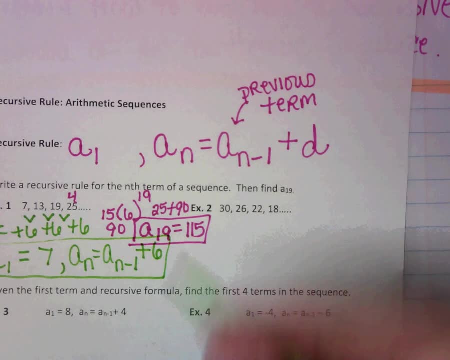 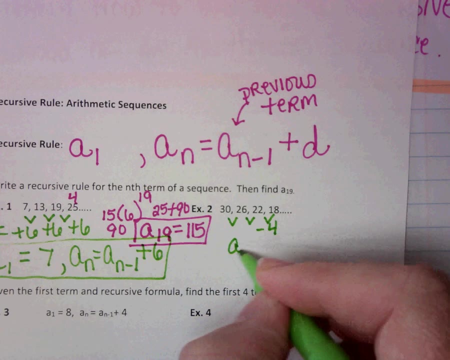 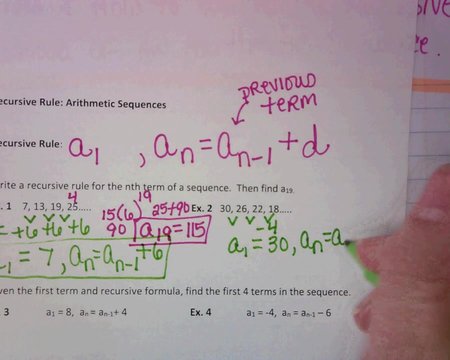 First thing we want to do is find the pattern. The pattern is that we are subtracting four every time, So we're going to state a sub one equals 30. And then we say a sub n equals a sub n minus one, minus four this time. 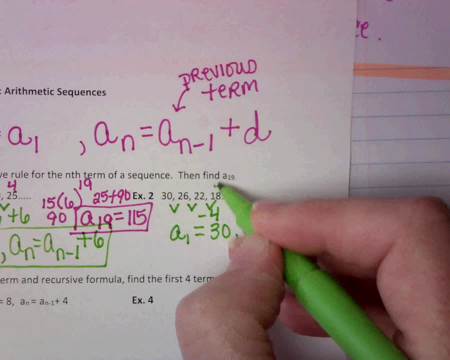 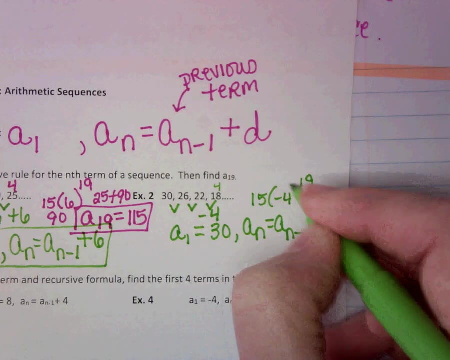 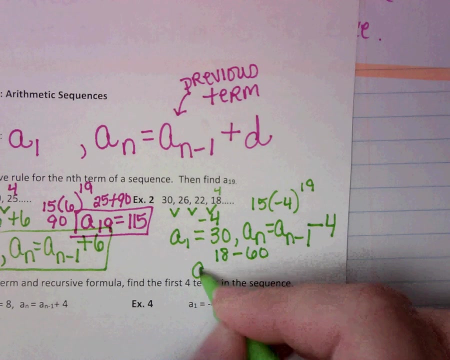 Okay. So we already said, we're trying to go to the ninth term, We're going to go to the sixteenth term. That's 15.. Fifteen times negative four is negative 60. So what is 18 minus 60?? 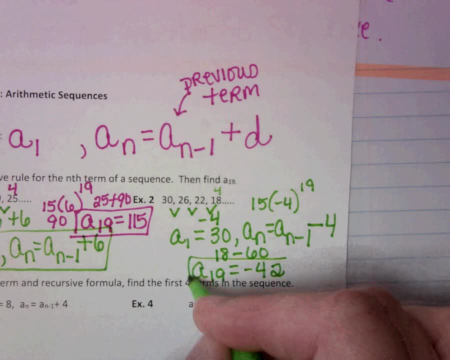 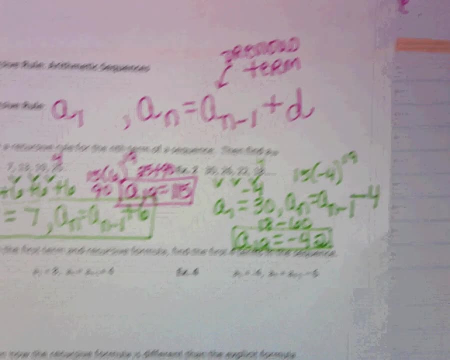 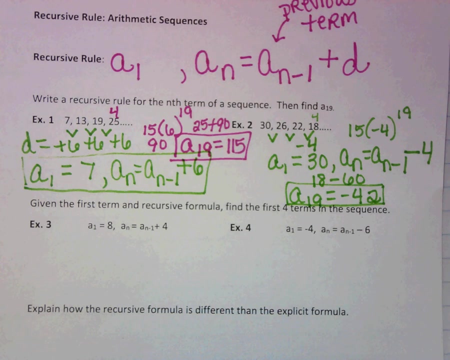 That would be negative 42.. A sub 19 would be negative 42.. Okay, Let's look at the next one. Find the first four terms in the sequence. I'm going to make it a little bit easier on you. The first term is eight. 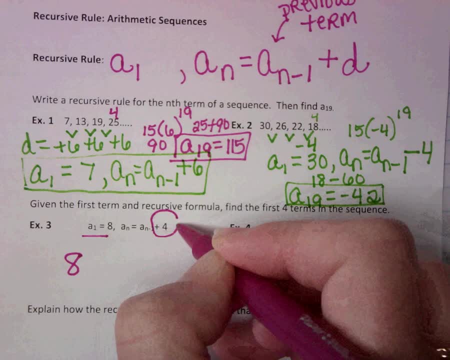 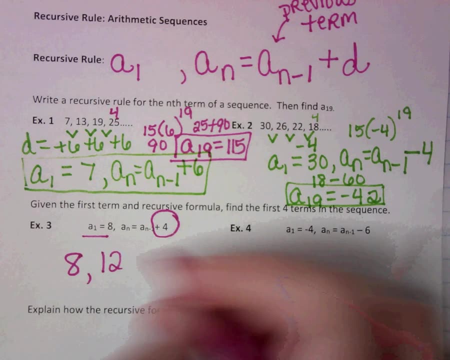 We should notice that the common difference is plus four. That's where the d goes. So if the first term is eight, we add four and we get 12.. We add another four, we get 16.. We add 20.. And there's the first four terms of the sequence. 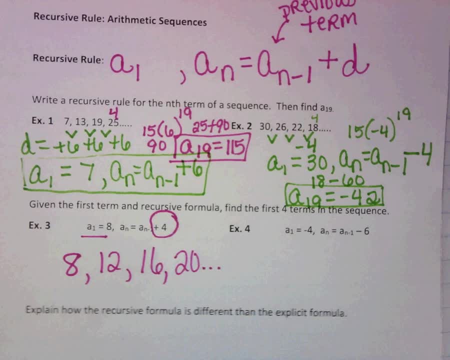 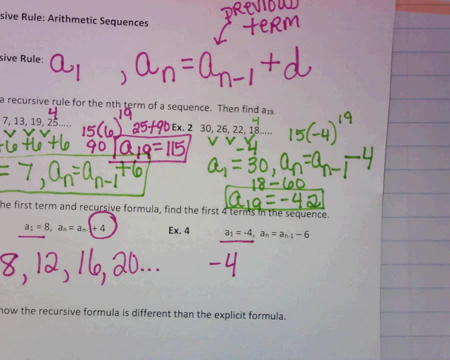 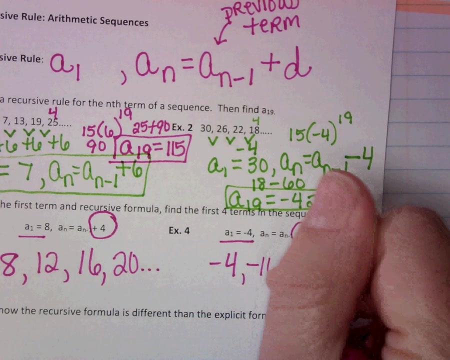 Super a lot easier, right? Okay, Look at the next one. First term is negative four. The common difference this time is negative six. So now I'm subtracting six, So negative four minus six is negative 10.. Minus six is negative 16.. 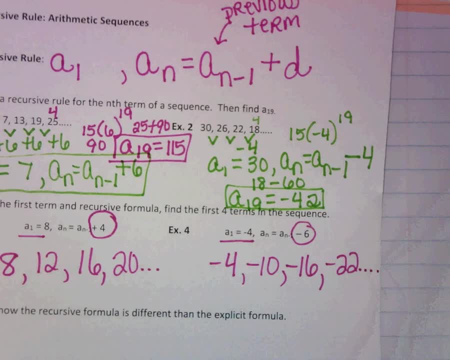 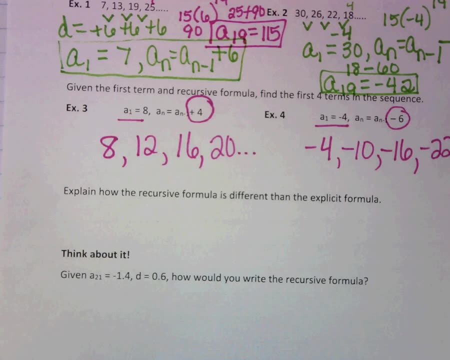 Minus six is negative 22.. Okay, The last two things on your notes here I want you to do for yourself, Okay, And we're going to talk about them in class tomorrow.